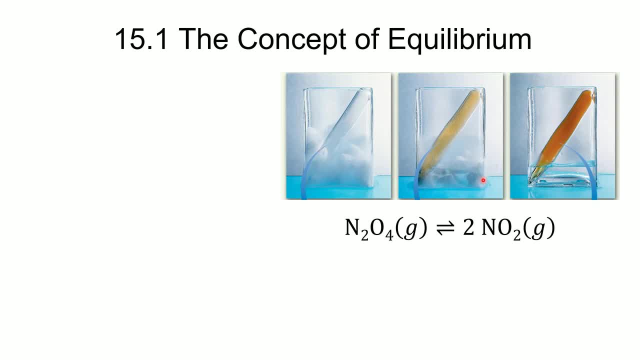 As we allow this to gradually warm up, and so here you can see that the reaction conditions have warmed up some. some of the NO2 is sublimated. We will find that the N2O4 will start to convert into a gas, and when it does, 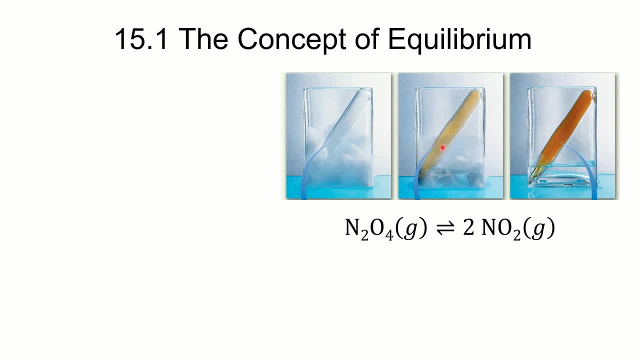 some of the N2O4 molecules will break apart to give us NO2 molecules. Well, the NO2 molecules have the distinct feature of being brown, whereas the N2O4 is completely colorless. So what we'll find is we can tell how much of the NO2 is present by how brown the mixture has gotten. 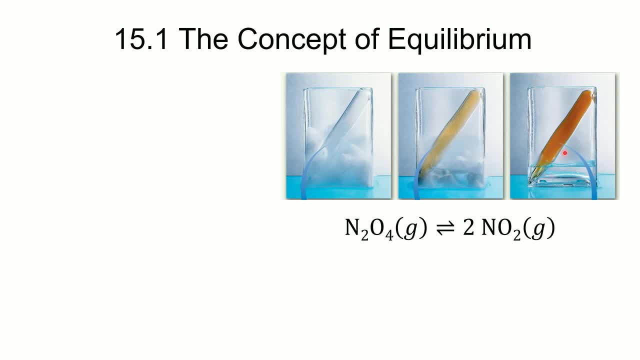 You'll see that once it gets up to room temperature, we will have significantly increased the amount of NO2, and therefore it is a much darker color. Well, we want to understand what are the conditions that are true when we get to equilibrium. 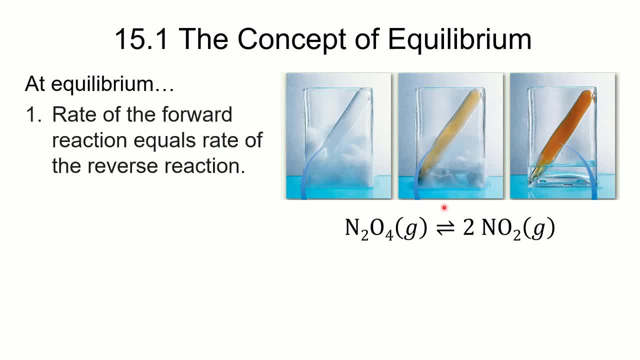 So one of the features of equilibrium is that the rate of the forward reaction is equal to the rate of the reverse reaction. So if we look at this particular equilibrium, we'll see that the rate of the forward reaction is going to be equal to kF times the concentration. 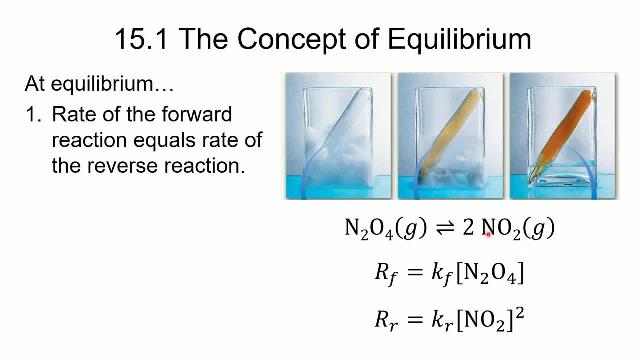 of N2O4 to the first power, The rate of the reverse reaction will be equal to kr times the concentration of NO2 squared, and that square of course comes from the coefficient. in the balanced equation We will find that at equilibrium R sub F will equal R sub R, And again that 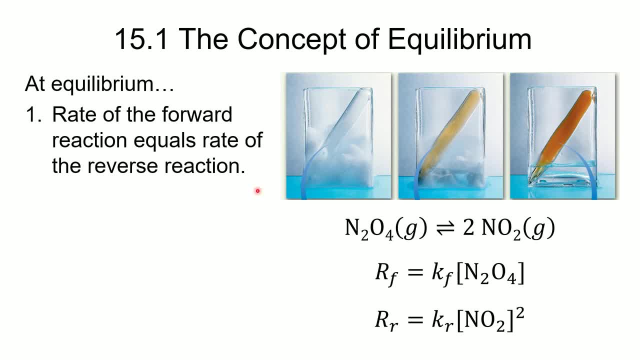 is one of the key features of equilibrium reactions. We'll also find that the concentration of reactants and products will remain constant at equilibrium, And I'll show you what that looks like here in just a moment. Finally, we'll see that the equilibrium ratio is constant once we get to equilibrium. So 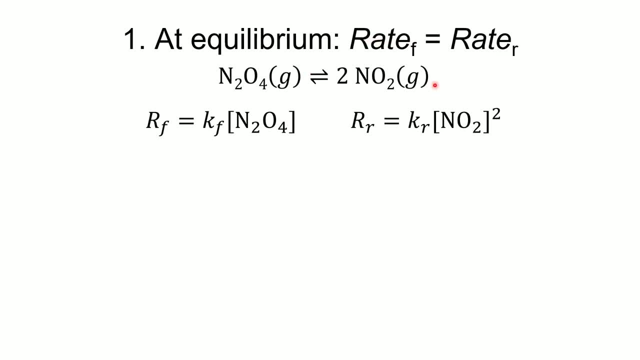 let's start with that first thing, that, yes, the rate of the forward reaction is equal to the rate of the reverse reaction when we get to equilibrium. So here, the rate of the forward is equal to the rate of the reverse reaction. And again, that is one of the key. 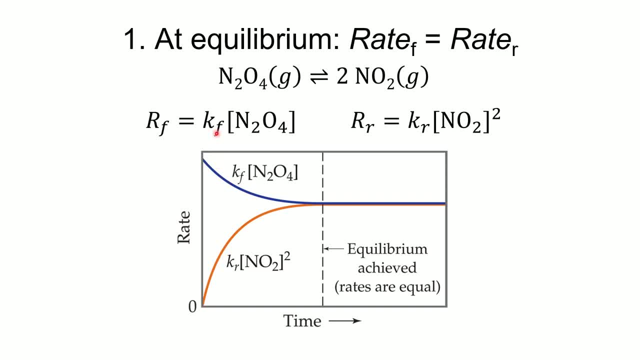 things Once again. the point is that if we were لكن was equal to kr times the concentration of NO2па, then kF would also be equal to kr times the concentration of NO2sta. In other words, n204 is equal to the frequency on the first power plus. 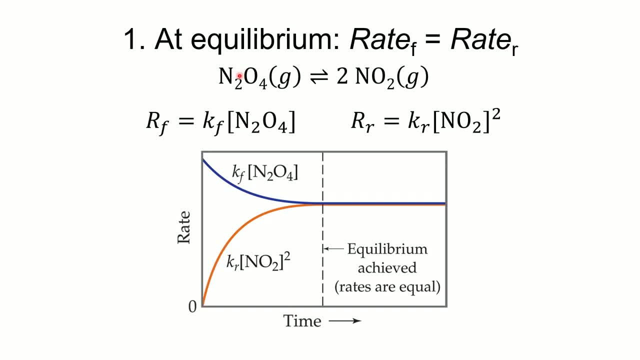 the 240, plus the rate of the forward reaction. Now there are a few siinä the rate of the forward reaction. that would be in the opposite direction. The number would be again darkened, that the weight of the forward possible carbon would not have accumulated. In this case with the bör, is like in a rough pastel, like a younger right side of a final step 3. ainsi, آmÉ bonds an, a 26e1n compared to ,9eMe would be also a姐 ài 옦žd. Sunday's recommendation of Kf times: the concentration of so you. 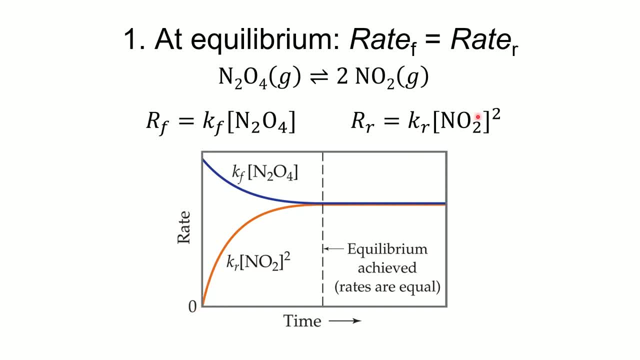 can show again in this example, and it onlyaro as candidates are intelligent really. As far as the reverse reaction goes, the rate of the reverse reaction would be equal to kr times the concentration of NO2 squared, And you'll see that since the concentration of NO2 started off at zero, that the rate 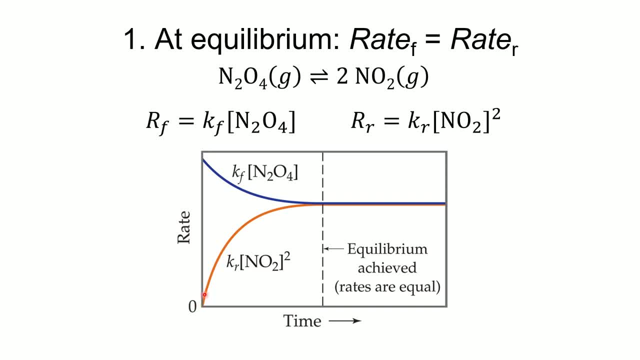 of the reverse reaction would have started off at zero as well and gradually increased as the concentration of NO2 increased. At the point at which the rate of the forward equals the rate of the reverse, we will find that the reaction is at equilibrium. 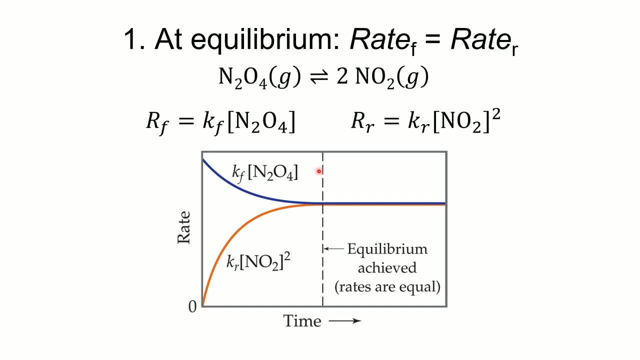 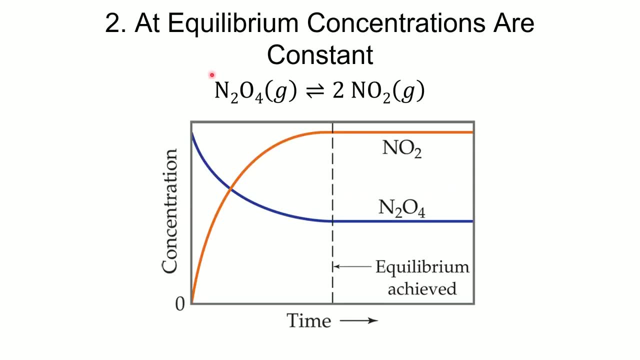 Both the forward and the reverse reaction are still occurring, but they are occurring at the same rate. As when we get to equilibrium, we'll also find that the concentrations will reach a constant value. As we mentioned earlier, the concentration of NO2 is at a constant value. 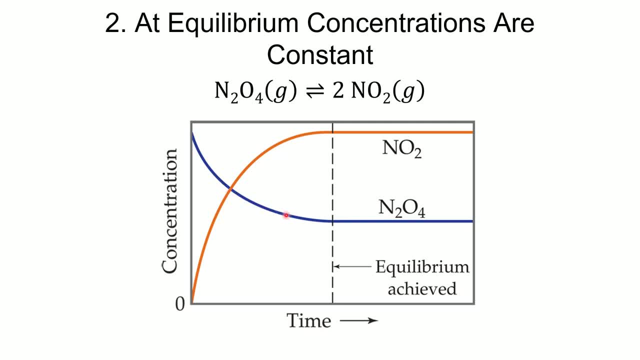 The concentration of NO2 would have started off relatively high and gradually decreased until it reached a constant value. The concentration of NO2 would have started off at zero, but it would gradually increase until it reached a constant value as well, And then, once they get to equilibrium, we'll see that they have reached a constant value. 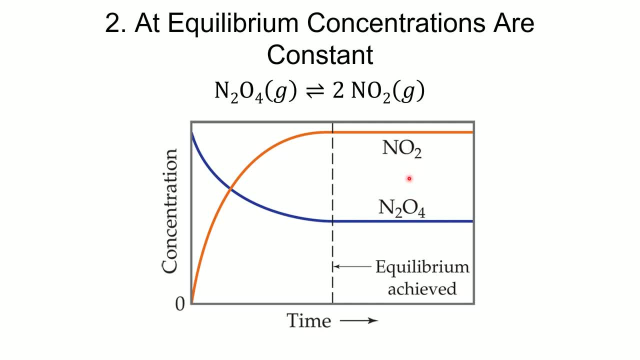 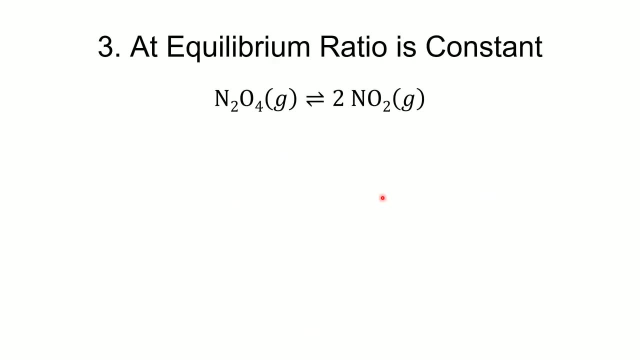 Note, however, that they are not necessarily equal to each other, And that is definitely not the case Here. they are not equal to each other. Finally, once we get to equilibrium, we'll find that the ratio of products over reactants. 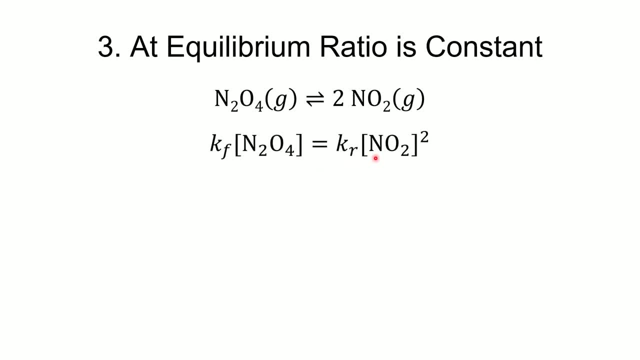 will be a constant value. So here the rate of the forward reaction equals the rate of the reverse reaction, as we discussed a little bit earlier. Well, we can solve this equation and get all of the constants over onto the left side of the equation by dividing both sides by kr. 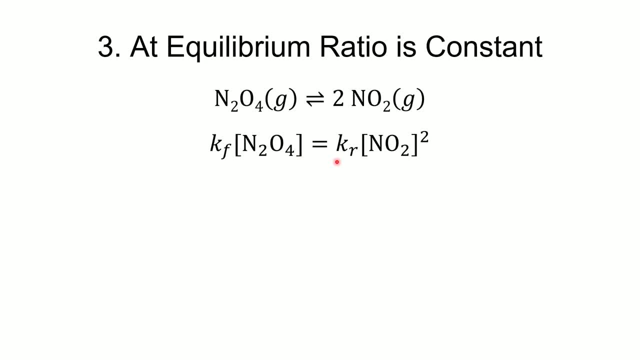 And get this. We get the concentrations over to the right side of the equation by dividing both sides by the concentration of N2O4. And that gives us this ratio. Well, if we take a constant and divide by another constant, we will get a constant. 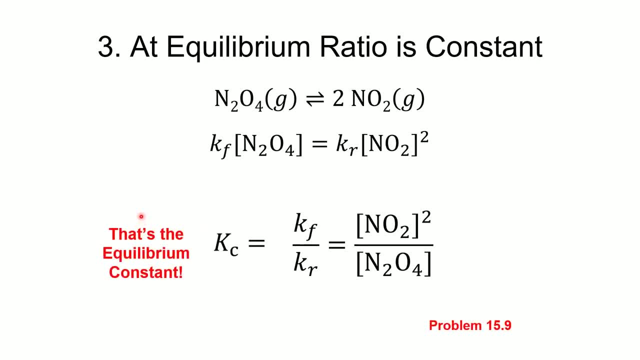 And that constant we will refer to as the equilibrium constant. We're going to talk about that equilibrium constant in more detail here in a few minutes, But suffice it to say that the rate of the reverse reaction is equal to the rate of the forward reaction. 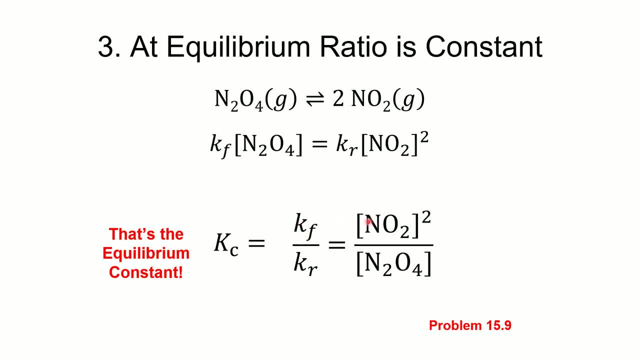 So we're going to get the concentration over to the right side of the equation by dividing both sides by kr, And that the concentration of our products divided by the concentration of our reactants will give us that equilibrium constant. So let's look at problem number 9.. 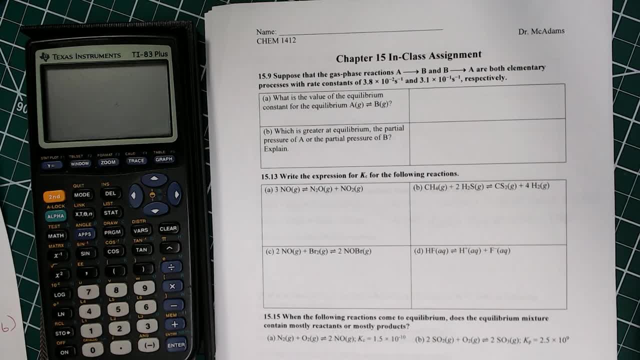 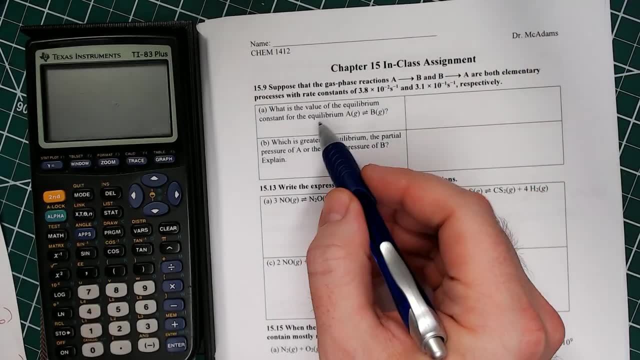 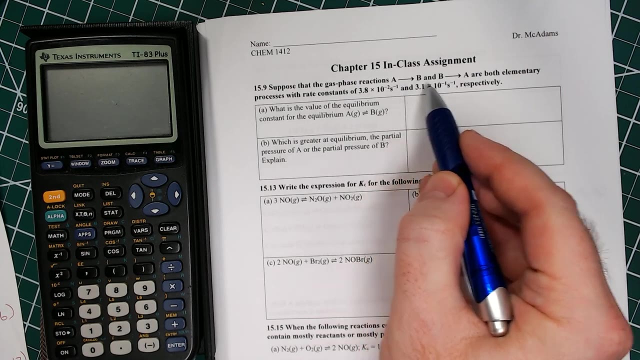 All right, so with problem number 9.. So with problem number 9.. what we want to do is we want to figure out what the equilibrium constant is for this particular reaction. So if we have a gas phase reaction where A is getting converted into B and B is getting converted into A, they have elementary 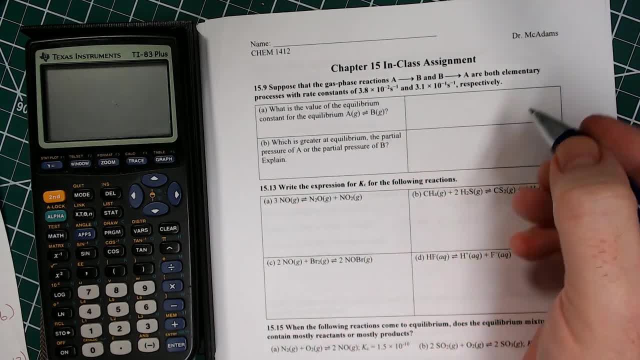 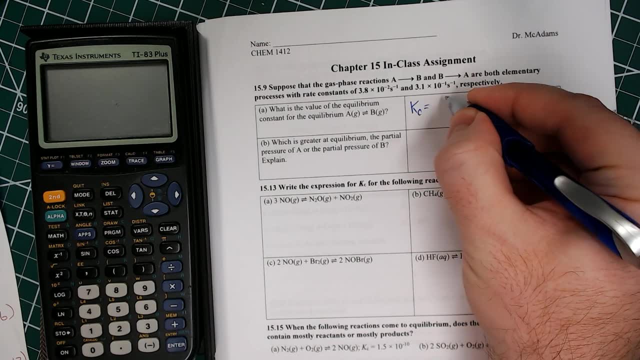 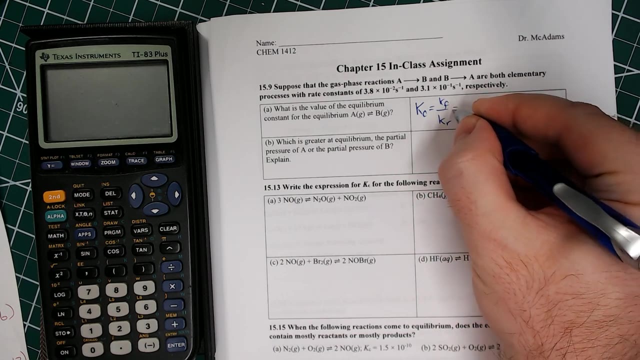 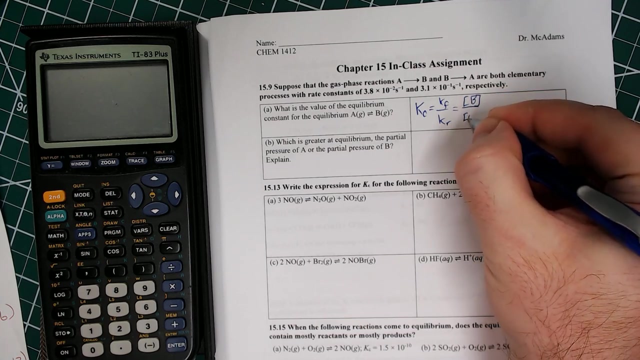 rate constants of these two values. Well, Kc is equal to, Kc is going to be equal to Kf over Kr, which is equal to the concentration of our product B over the concentration of our reactant A. We know that the value of 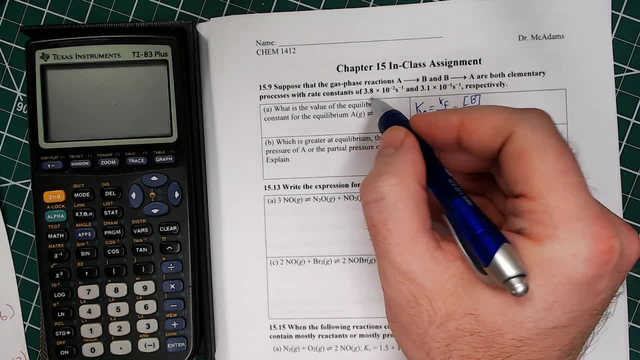 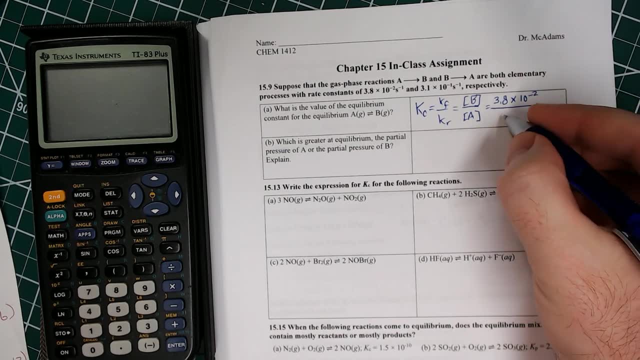 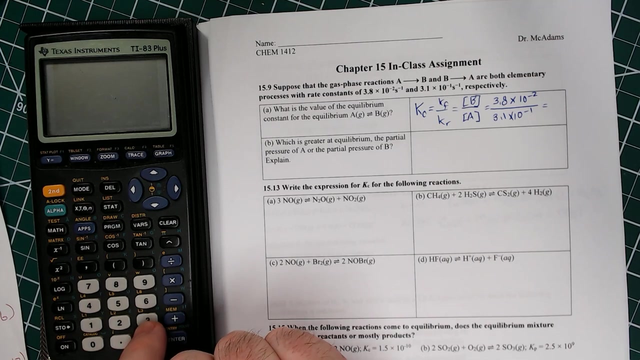 Kf and Kr are given here, so 3.8 times 10 to the negative 2, and for the reverse reaction, 3.1 times 10 to the negative 1.. Well, with that we can easily calculate our equilibrium constant Kc. 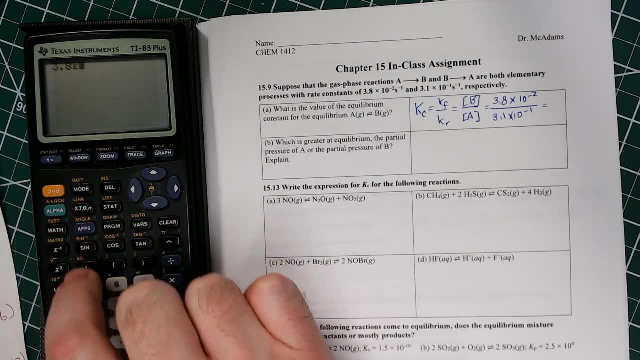 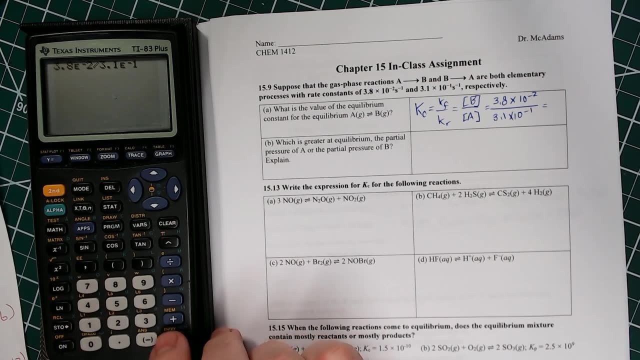 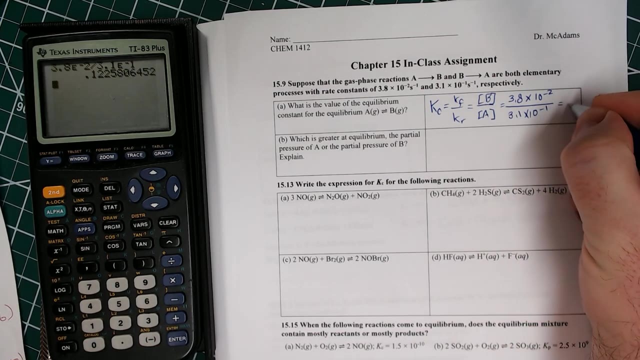 3.8 times 10 to the negative 2, our equation will have: and then divide that by 3.1 times 10 to the negative 1.. And that gives us 0.1226.. We're going to round that to two significant figures. 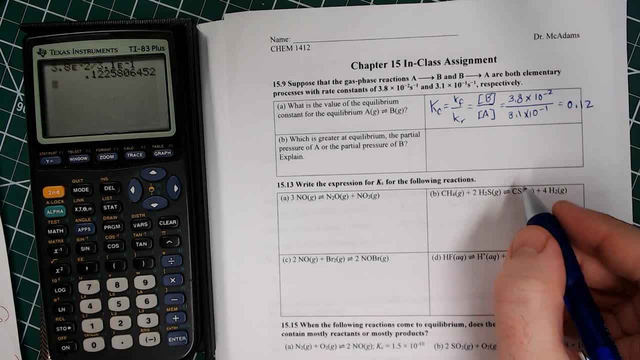 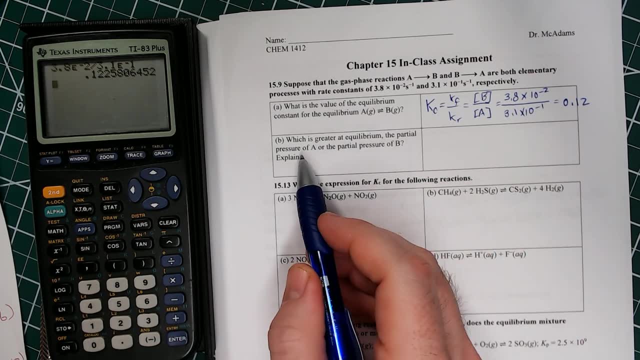 so we'll put 0.12.. So that would be our equilibrium constant for this particular reaction. Well, the question here in part B: which is greater at equilibrium, the partial pressure of A or the partial pressure of B? Now here we've got the concentrations of A and B. 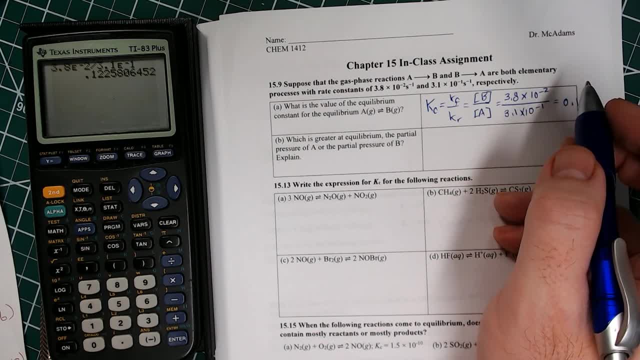 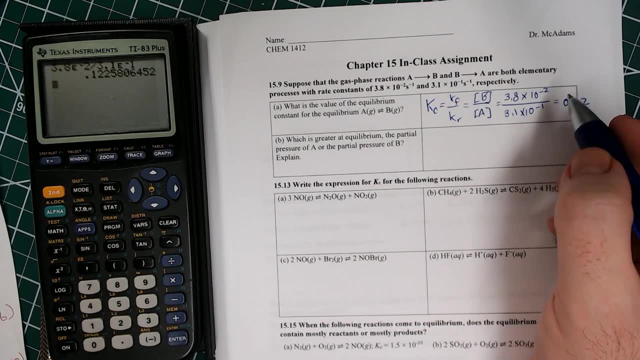 but since concentration is proportional to the partial pressure, we can use the values that we have here to answer this question. So you'll notice here that the ratio of B to A is going to come out to 0.12.. That means that we have more of A than we do of B. 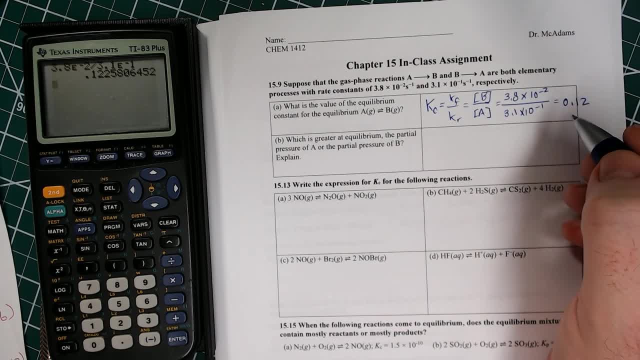 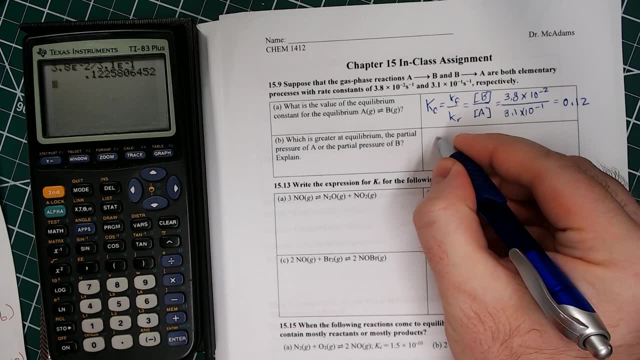 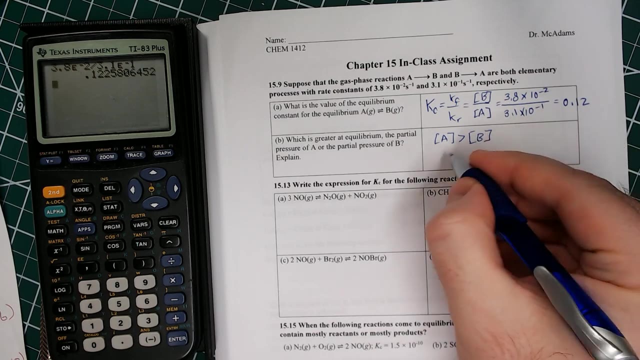 About 8 times as much of A as we do of B. Well, if we have 8 times as much of A as we do of B, that means that the concentration of A is greater than the concentration of B. That also means that the partial pressure of A 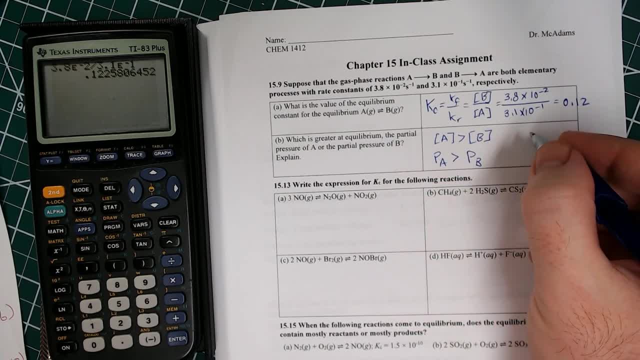 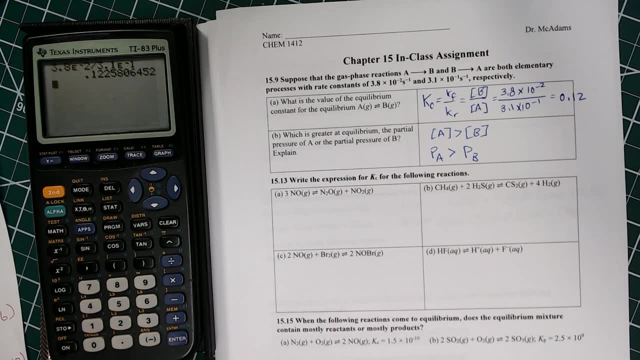 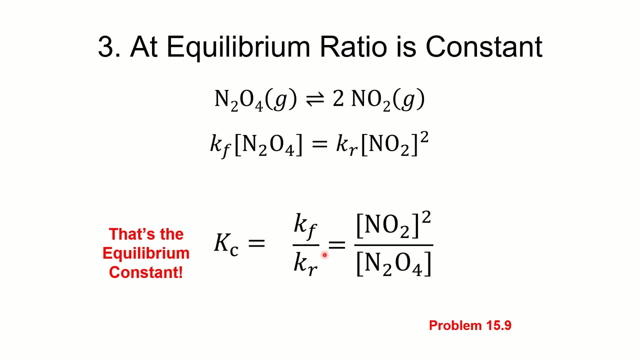 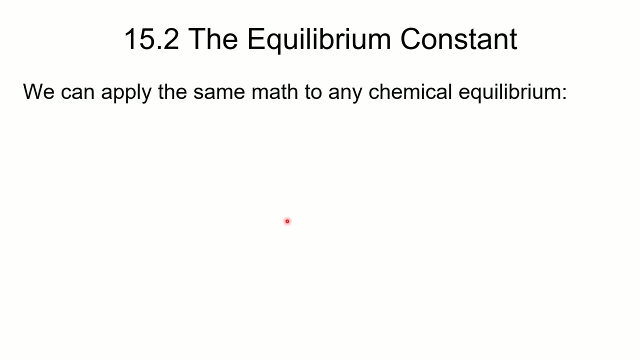 is going to be greater than the partial pressure of B. All right, So now we're going to switch back And we want to look at something that we refer to as the equilibrium constant, So we can apply the same math to any kind of chemical equilibrium. 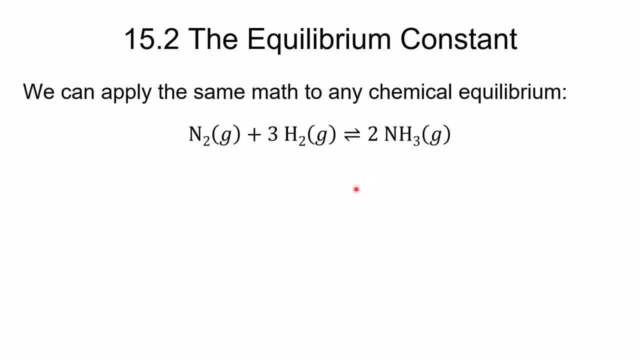 For example, for the reaction between nitrogen and hydrogen to give us ammonia, which is a very important product. it's a very important process that we will be discussing later in this chapter. We'll find that the rate of the forward is equal to Kf times the concentration of N2. 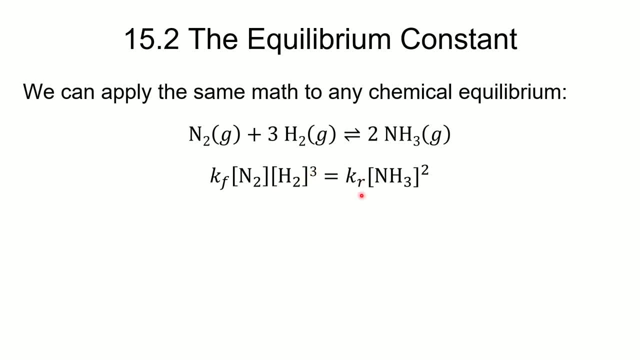 times the concentration of H2 cubed. The rate of the reverse is equal to Kr times the concentration of NH3 squared. And again, that square comes from the fact that the coefficient is 2.. Well, here we can write again: solve for Kf over Kr. 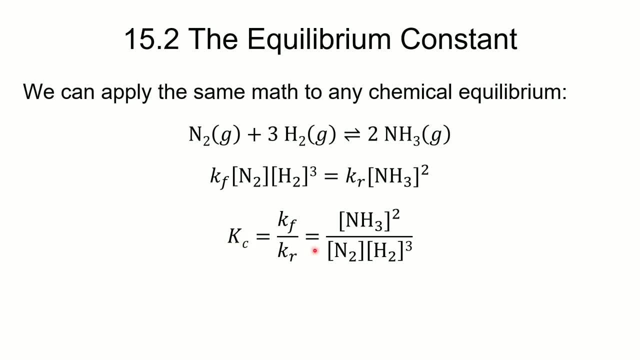 and that will give us our equilibrium constant Kc And we will have our concentration of ammonia squared, divided by the concentration of N2 and also divided by the concentration of H2 cubed. If we want, we can generalize this. This is our equilibrium constant expression. 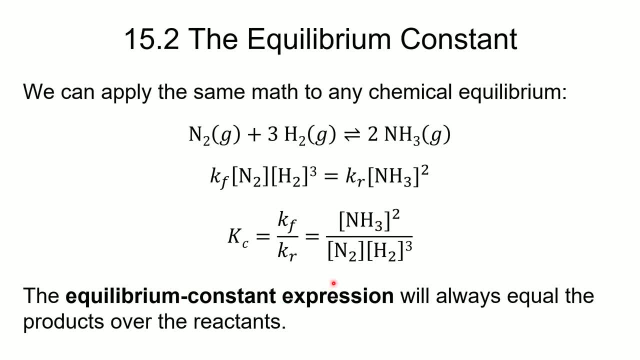 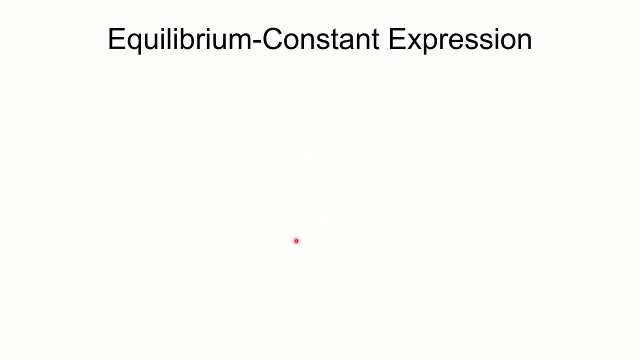 It'll always be products over reactions, And we can generalize this for any value for these coefficients. So for A, B, C, whatever. So here is a generic form of the equation, where the lowercase letter represents the coefficient and the uppercase letter represents the chemical. 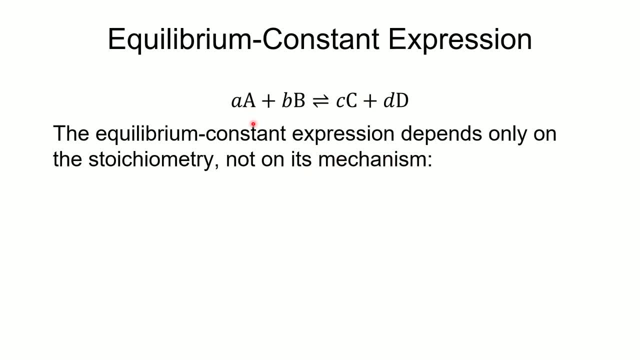 The equilibrium constant expression will only depend on the stoichiometry, In other words, it will only depend on those coefficients. It does not depend on the mass, It only depends on the mechanism. So here is our equilibrium constant expression. Kc equals the concentration of C raised to the C power. 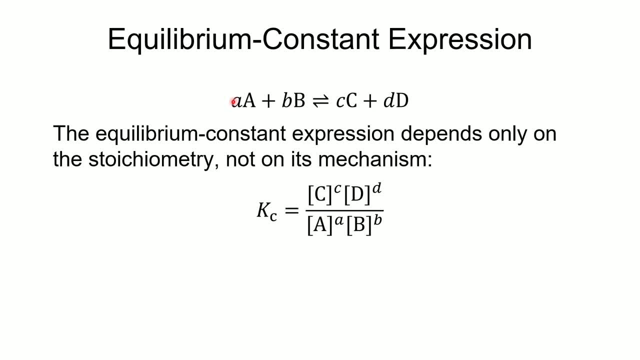 concentration of D raised to the D power, divided by the concentration of A raised to the A power and concentration of B raised to the B power. Note that when you're using Kc, your equilibrium constant expression, written using concentrations in molarity, We will see here in a few minutes we're. 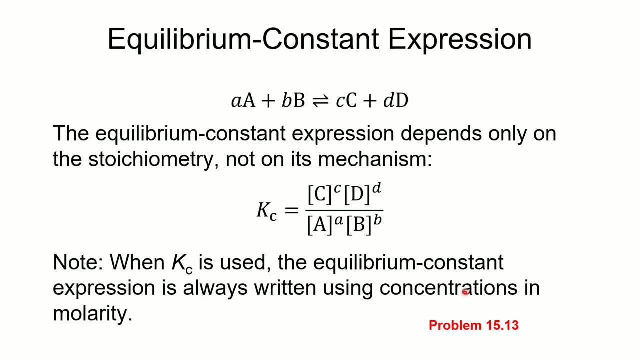 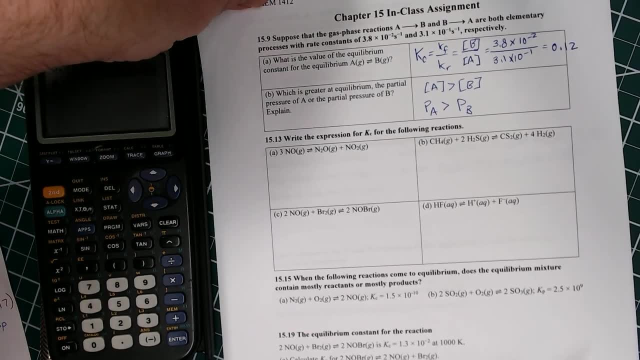 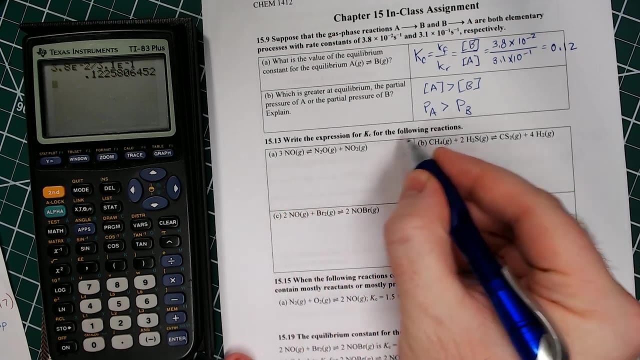 going to use one version where it's written in partial pressures, but that will be here in just a few minutes. First let's look at number 13 on the in-class assignment. Alright, so here we want to write the equilibrium constant expression for each of these. We are writing it in terms of kC, So kC is. 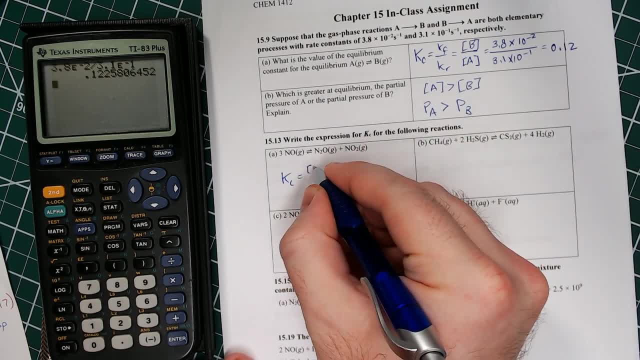 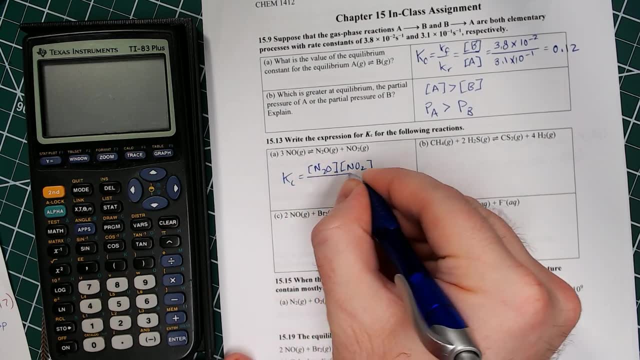 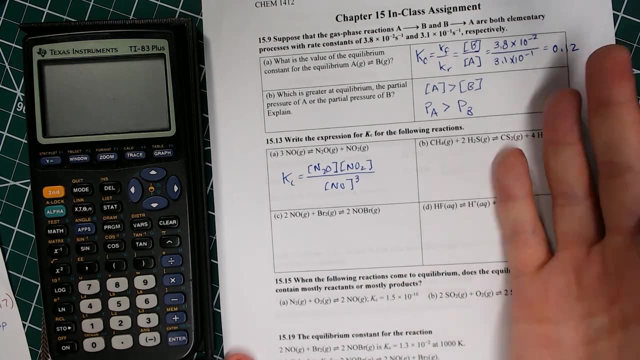 equal to products over reactants. so we'll put NO2O times the concentration of NO2.. Then we'll divide that by the concentration of NO3.. Now we don't know what the value of kC is. here we're just writing out the. 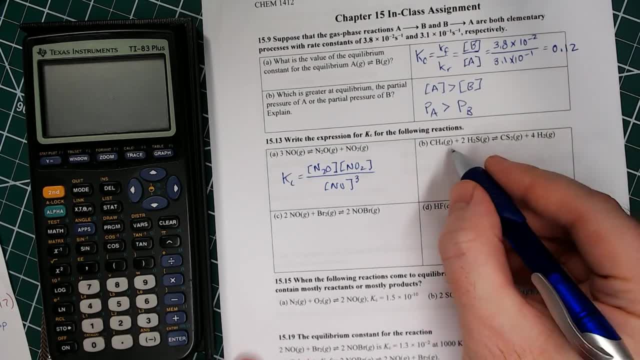 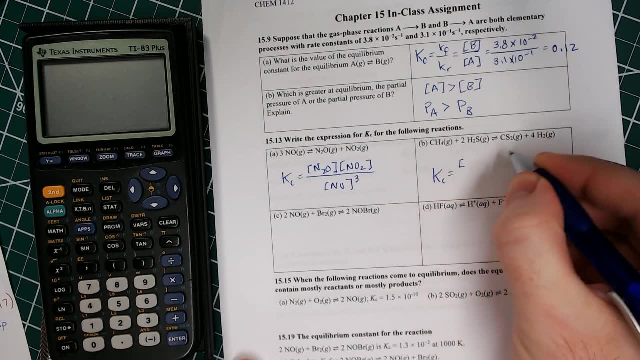 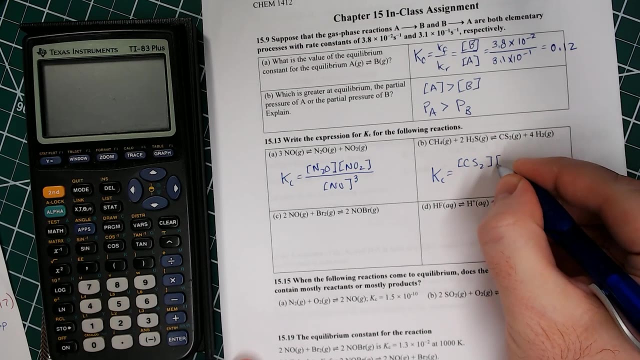 expression In Part B we will see again. just follow the stoichiometry. so products over reactants. So here we've got concentration of CS2 raised to the first power. Of course we don't need to put the 1.. 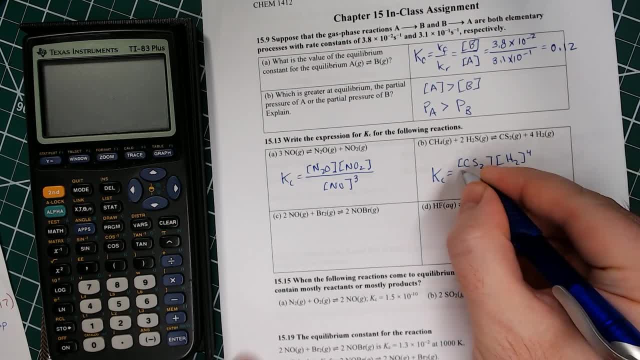 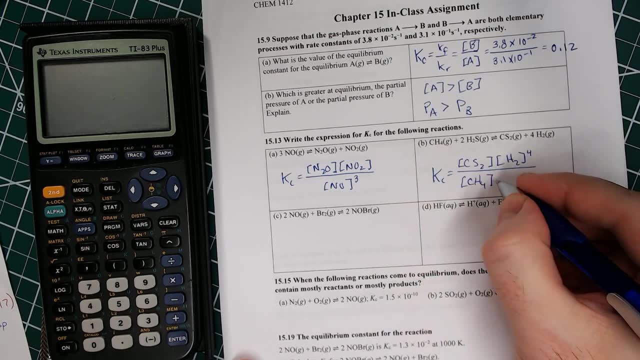 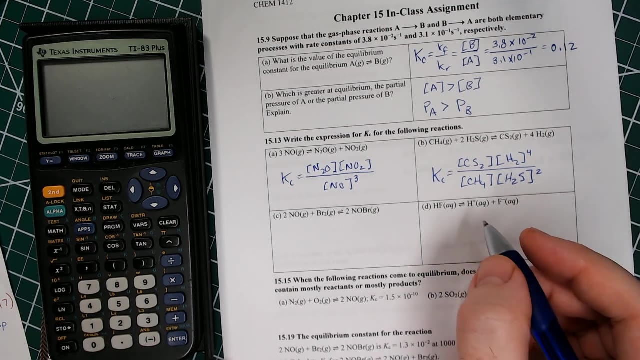 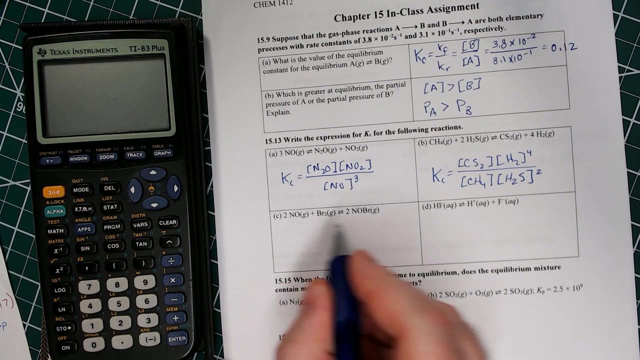 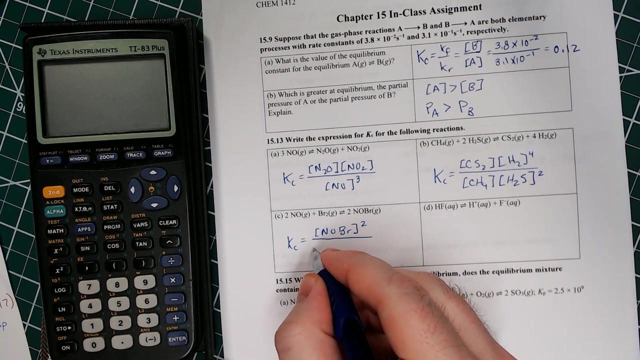 Concentration of H2 raised to the fourth power, divided by the concentration of CH4 raised to the first power, times the concentration of H2S squared And that gives us our equilibrium constant expression. Alright, for this one. KC is equal to the concentration of NOBr2 divided by the concentration. 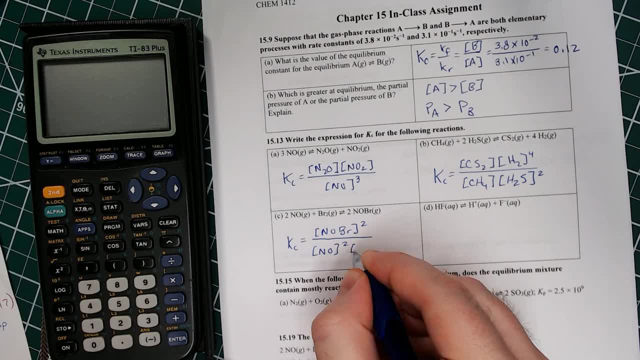 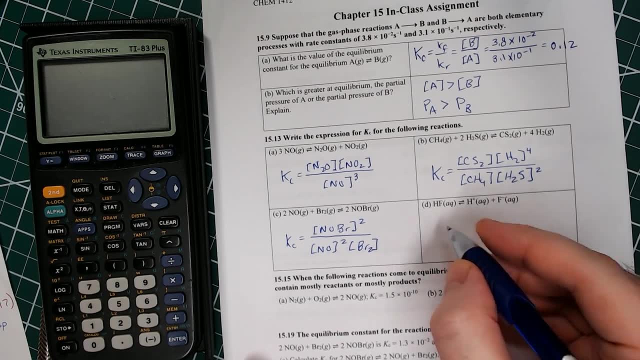 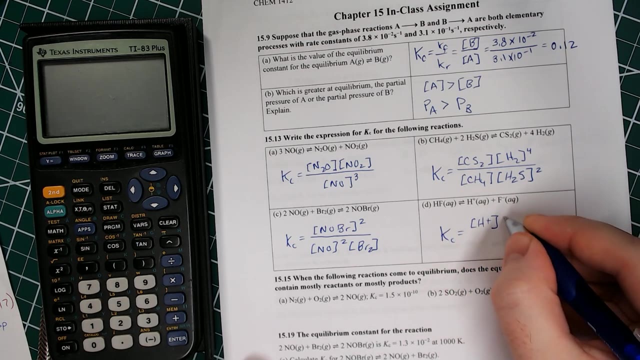 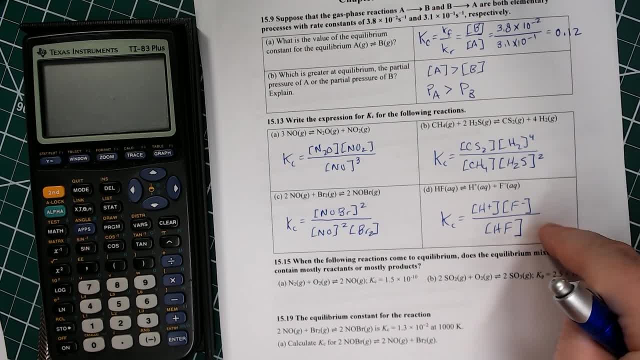 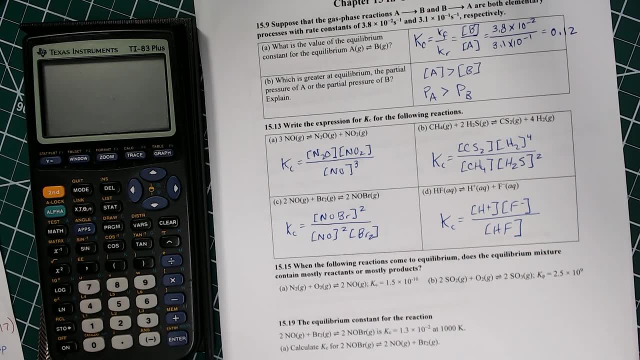 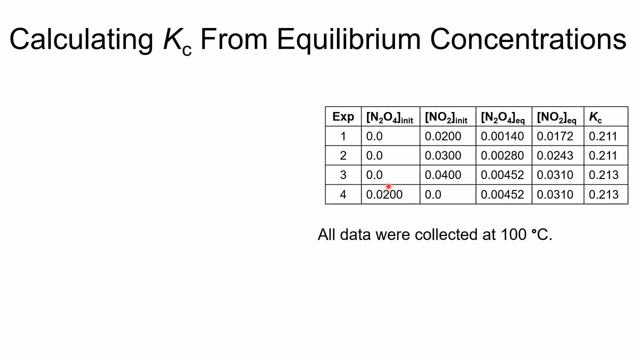 course of this chapter. so you want to get good at writing out equilibrium constant expressions, Alright, so now on to the next topic. So it's possible to calculate the value of KC from equilibrium concentrations. And so, when calculating the value of KC from the equilibrium concentrations, we're going 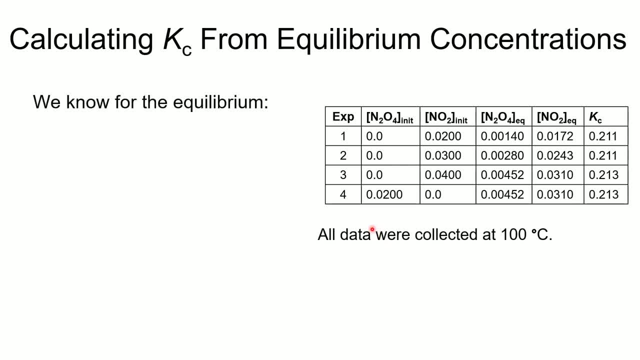 to need to calculate the value of KC from the equilibrium concentrations. We just need to go over and look at what the equilibrium concentrations are. Now, here we've got four different experiments that started off with different amounts, initially of the N2O4 and NO2.. 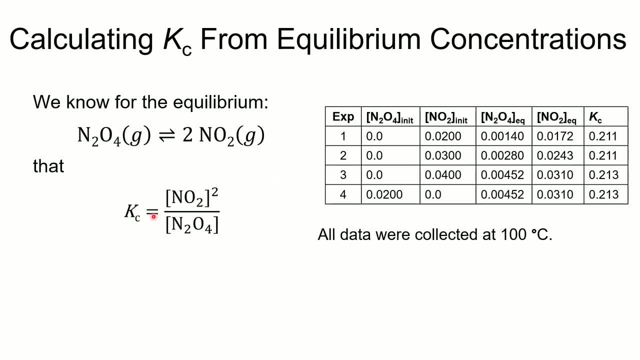 And we know that this is our equilibrium- constant expression- and we simply need to take the values from any of these experiments. So we're going to take the values from any of these experiments and we're going to take the values from any of these experiments and we're going to take the values from any. 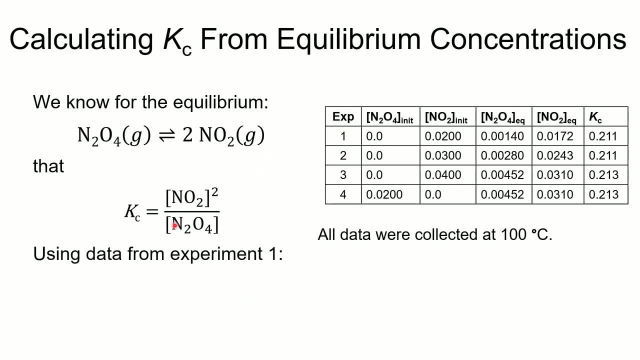 of these experiments and we're going to take the values from any of these experiments. We're just going to use experiment one to start with And we put the number in. so the concentration of NO2 is equal to 0.0172 molar. 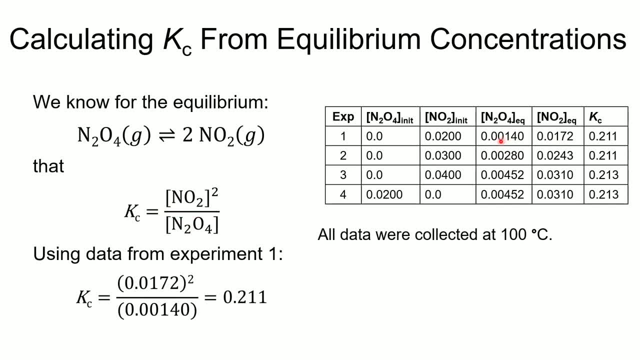 The concentration of N2O4 is 0.00140.. And then when we do that number, squared over this number, we will get the value of 0.211.. 0.211. 0.211.. Now we will find that we're going to leave Kc as a unitless number. 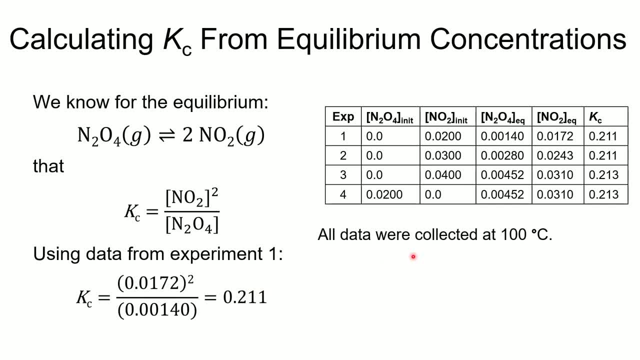 Even though technically there are units, we're going to write it as a unitless number And then, if we do the same experiment with several other initial concentrations, instead of starting with 0.02 molar NO2, we can start with 0.03, 0.04.. 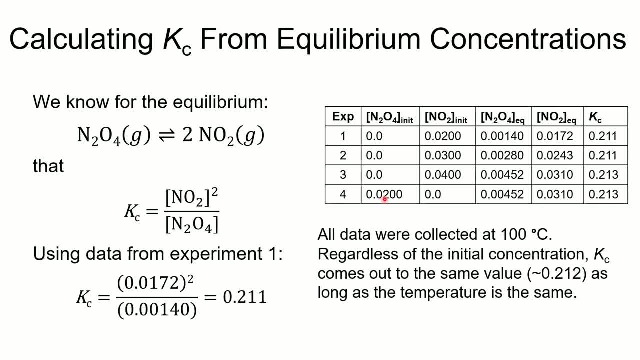 0.03.. 0.04.. 0.04.. And we can even start with 0.02 molar N2O4 and none of the NO2.. Regardless of which one of those we get, we get approximately the same value. 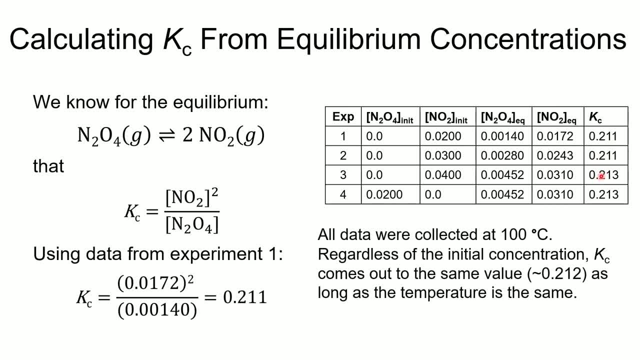 On average, these come out to 0.212 as our value for the equilibrium constant Kc. As long as the temperature is the same, we will get the same value again within experimental error: 0.212.. 0.212.. 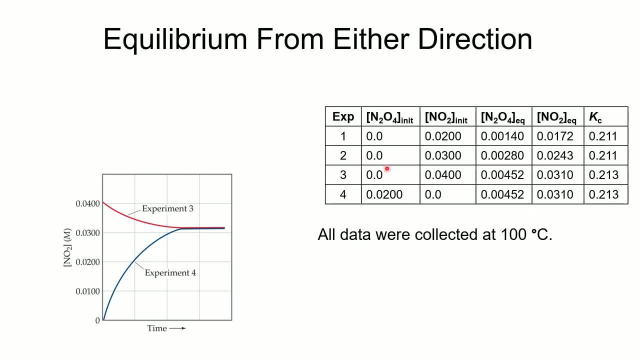 0.212.. 0.212.. from either direction. If we look at experiments 3 and 4, in experiment 3 we started off with none of the N2O4 and 0.0400 molar NO2.. Well, the 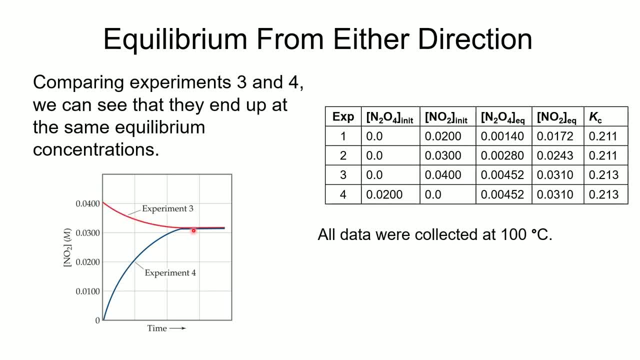 concentration of NO2 decreased as time went on and eventually reached a constant value. That constant value came out to 0.0310 molar for the NO2 at equilibrium and, of course, the concentration of N2O4 increased. If we look at the data in experiment 4, you'll see that the concentration of NO2 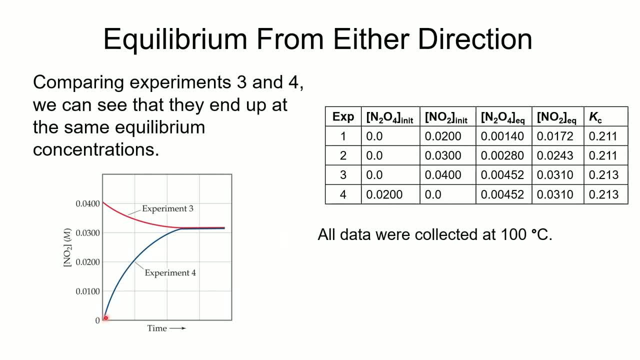 started off at 0, so here it is at 0.. As time goes on it would increase, and that's because the concentration of N2O4 started off at 0.0200 molar. Well, we would find that concentration of NO2 would increase to the. 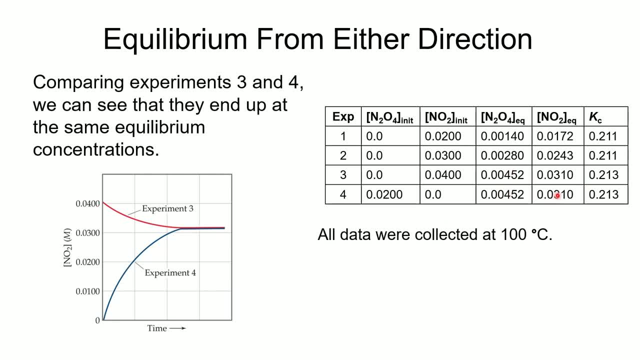 same amount. In fact, we would get exactly the same concentrations for N2O4 and NO2 in experiments 3 and 4.. In fact, if you were to set up both of these experiments and not label them and then have somebody else come into the 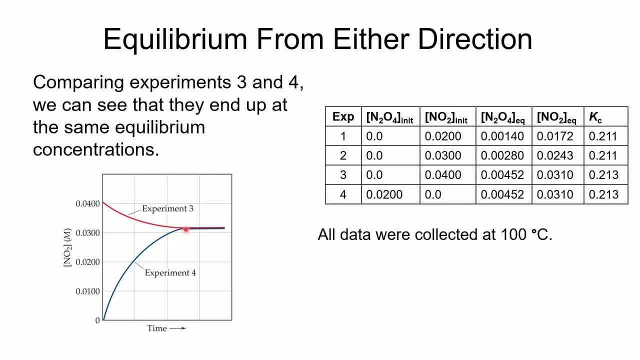 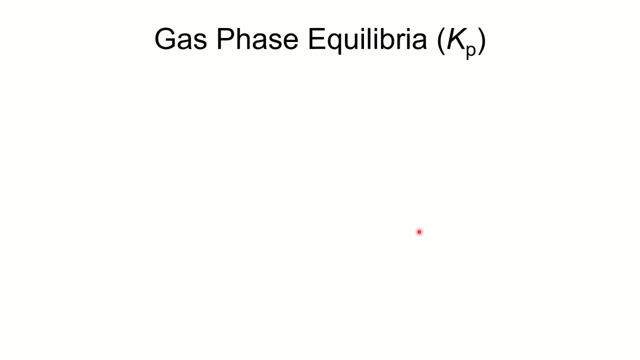 room after some amount of time, you would find that they would not be able to tell which one was experiment 3 and which one was experiment 4, because they would have exactly the same concentration. For gas phase equilibrium we can write a different kind of equilibrium constant. 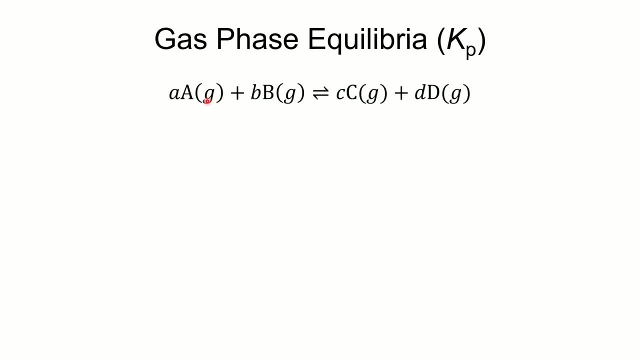 and that different kind of equilibrium constant depends on everything being in the gas phase. If there's something that's not in the gas phase, this doesn't really work very well. But if everything is in the gas phase, then we can write an equilibrium constant. 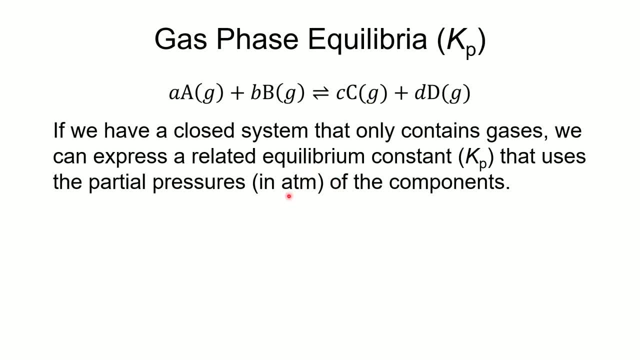 We can write an equilibrium constant, Kp, where instead of using molarities we can use partial pressures in atmospheres. And so here we've got: Kp is equal partial pressure of C, again, products over reactants, and we're using partial pressure of C raised to the C power. 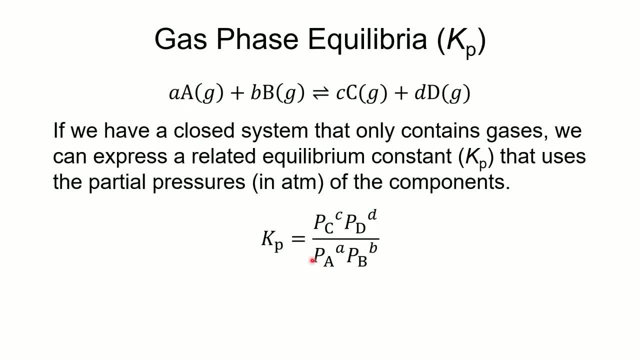 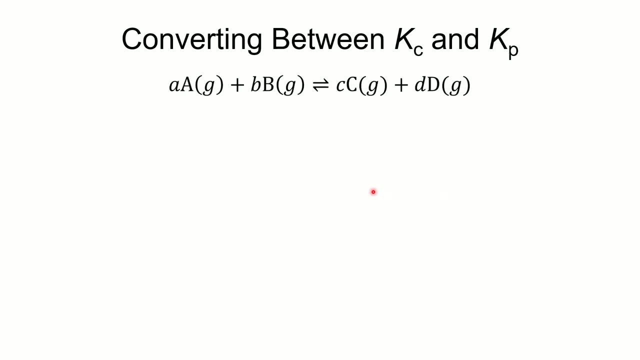 partial pressure of D raised to the D power over partial pressure of A raised to the A power and partial pressure of B raised to the B power. If we want to get the relationship between Kc and Kp, that's relatively easy to do. 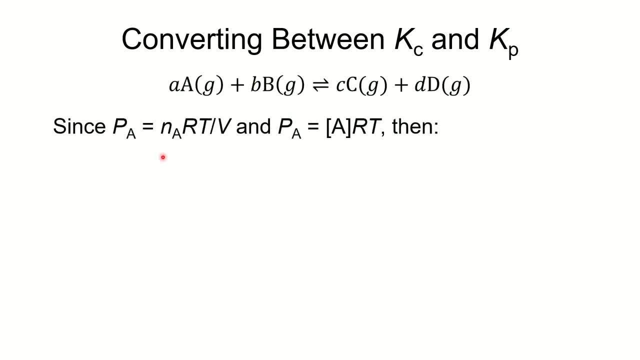 So again, here is the equation. We know from the ideal gas law and from Dalton's law of partial pressure that we can write, using the ideal gas law, that the partial pressure of A is equal to the number of moles of A times the gas constant, R times the temperature. 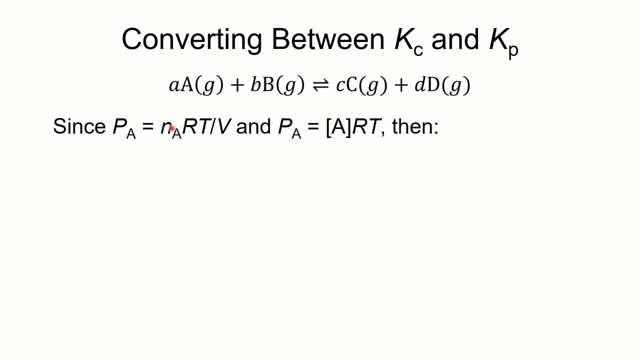 in Kelvin divided by the volume. Since the number of moles divided by the volume is equal to the concentration, then the partial pressure of A is equal to the concentration of A times RT. Well, given that we can rewrite these partial pressures in terms of the concentrations times, 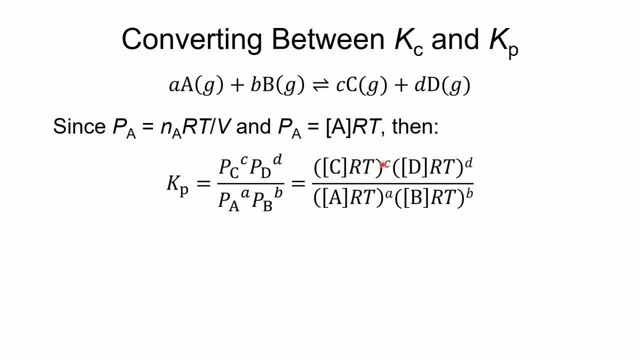 RT and raise to whatever their coefficient is as the exponent. Well, since R and T are going to be the same for all of these, we can factor out R and T and get this. So when we factor out R and T, we'll get R times T raised to the C plus D on top, and 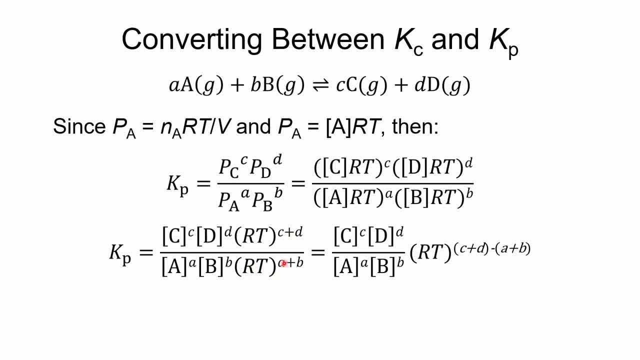 down in the denominator, we'll get RT raised to the A plus B. We can combine these terms. we'll do the numerator value here minus the denominator and we will get R times RT. RT raised to the C plus D, minus parentheses: A plus B. 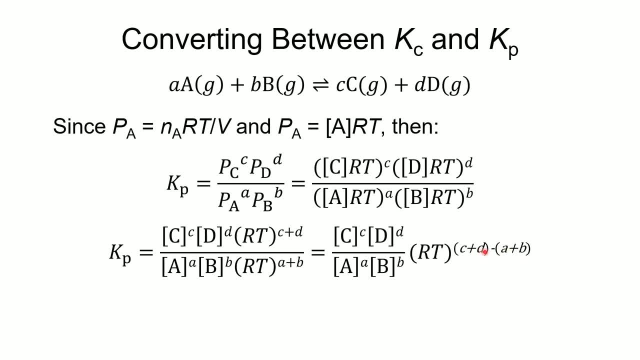 Well, this is the change in the number of moles of gas. Since this part is equal to KC, we can now get that KP is equal to KC times RT raised to the delta N power, Where delta N is the number of moles. 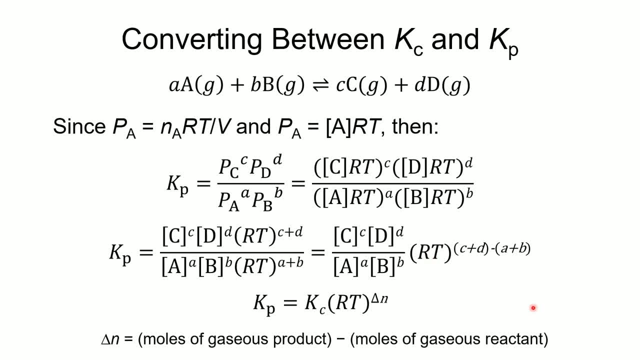 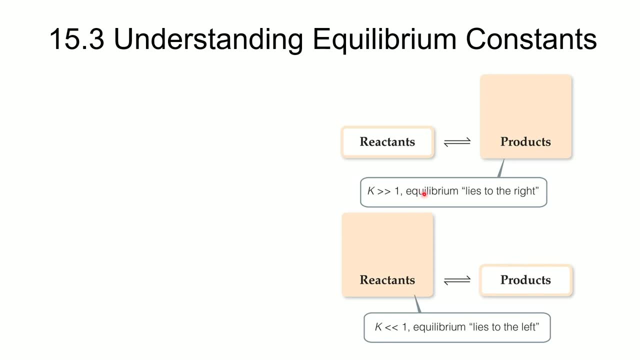 So we can get the number of moles of gaseous product minus the number of moles of gaseous reactant. We will do an example of this here in just a bit. All right, Well, now we want to look at what the equilibrium constant value actually means. 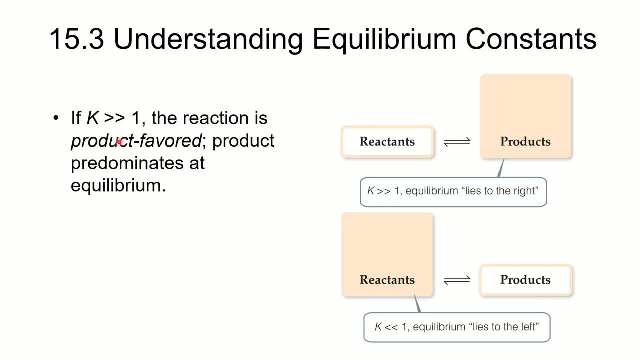 So we're going to start by looking at if KC is a variable. If K is a very large number, or K is a very large number, it's much greater than 1, then that means that the reaction will be product favored In terms of what do we have more of? if K is greater than 1, we should have a lot more. 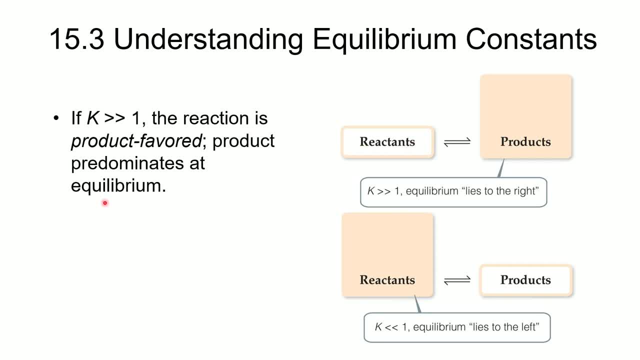 of the product than we do of the reactant. If K is much less than 1, we generally say that the reactant or the reaction is reactant favored And that that reactant will predominate. Okay, And so we have a lot more reactant at equilibrium.